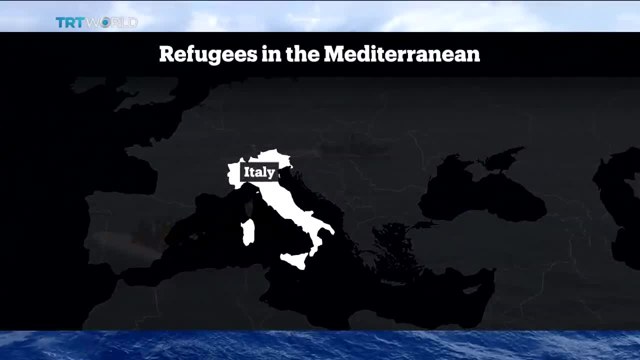 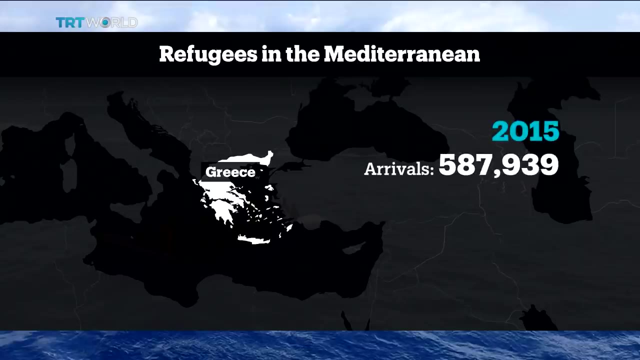 Between January and November the 17th last year, almost 141,000 people arrived in Italy. That's compared with 167,000 for the same period this year. In the meantime, arrivals in Greece have gone down from 587,000 in 2017 to 167,000 this year. But the number of deaths are still rising: 3,541 in 2015,, but already there have been 4,559 since January. There's one big reason why so many refugees like these didn't end up in Greece: They're now sent back if they don't claim asylum or have their claims rejected because of a deal. 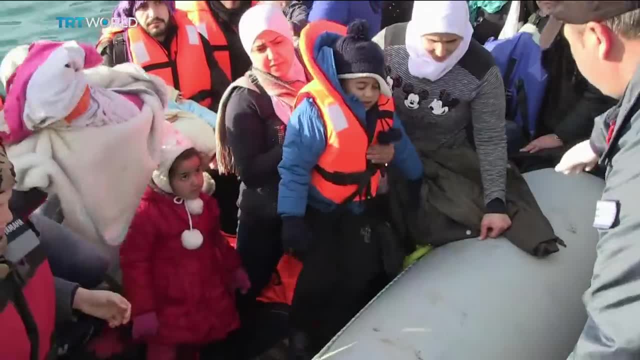 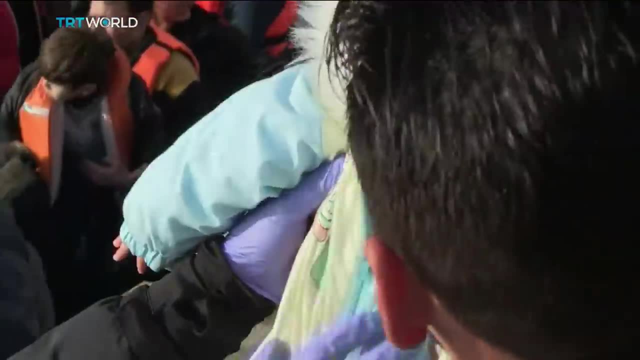 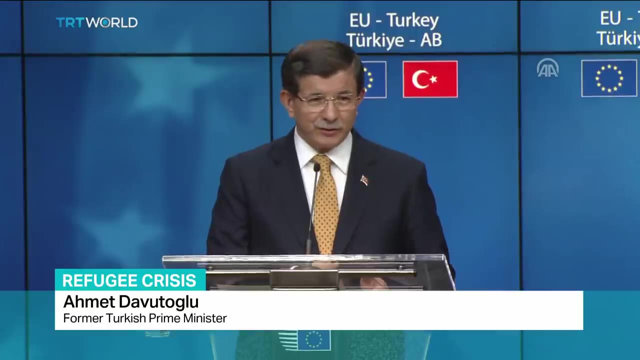 in March between Turkey and the EU. It's appeared close to collapse at times due to disputes over its exact terms, but was hailed a triumph. We shared our views, we shared our concerns, we shared our perspectives and vision And we today realize that Turkey and the EU have the same destiny, the same challenges and 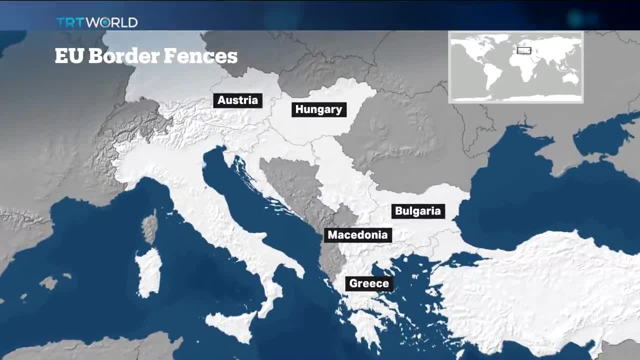 the same future, But it seems the shared vision for many in the EU is to build fences along their borders. Refugees now have them or are putting them up. well over 1,000 kilometers: Greece, Bulgaria, Hungary, Austria, Macedonia, And there could be more in the pipeline. 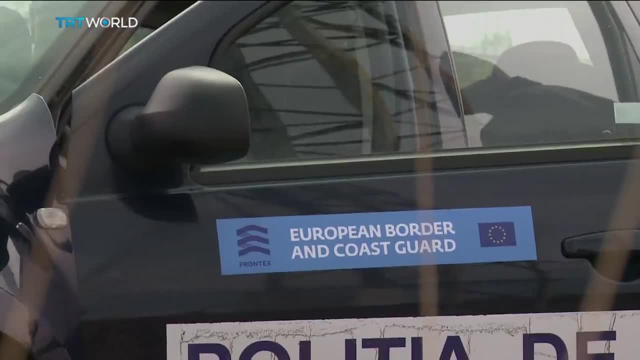 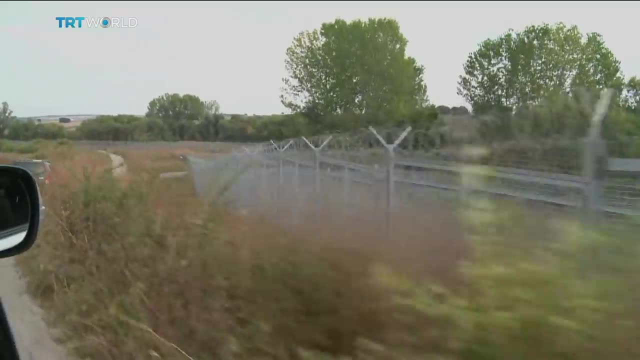 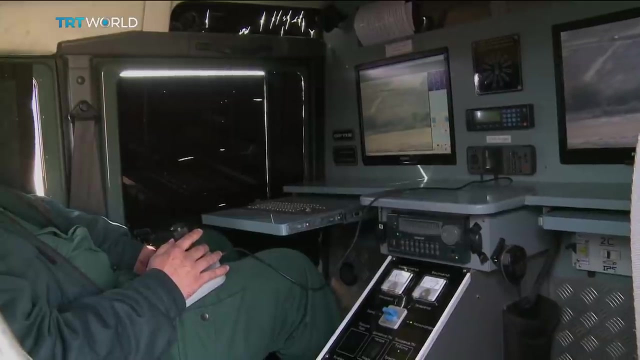 The emphasis for many of these countries seems to have been how to keep the refugees out. A new EU border police and coast guard force was launched, And a scheme to resettle 160,000 refugees by the EU has been quietly kicked into the long grass, As members stated. 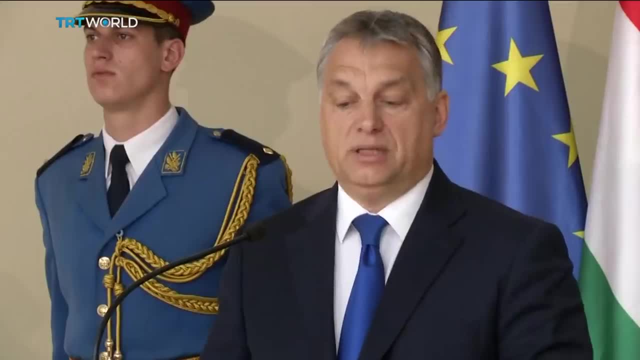 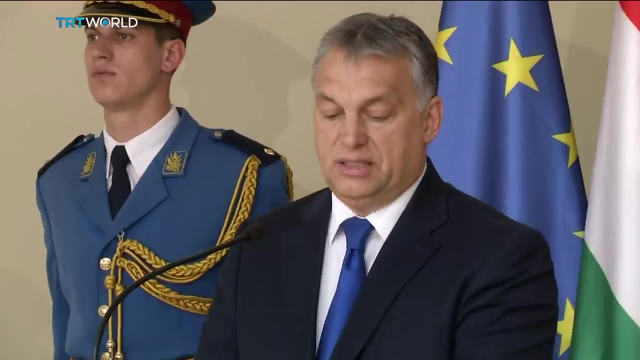 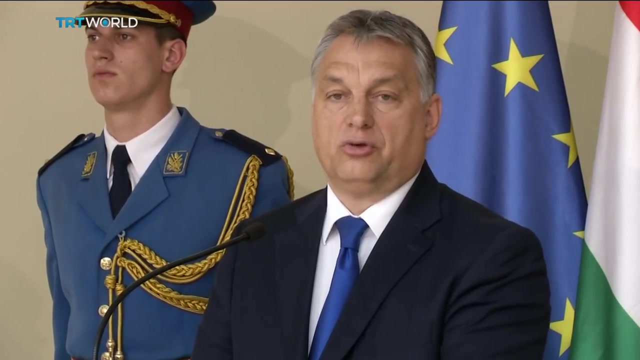 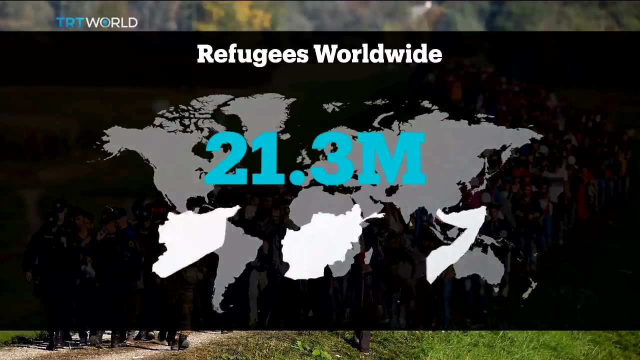 The United States showed a distinct lack of enthusiasm. Hungary will do everything to return every migrant from Europe to their home country And Hungary will do everything to prevent anyone from entering and staying illegally, violating Hungarian laws. The UN says there are more than 21 million refugees worldwide, More than half from just 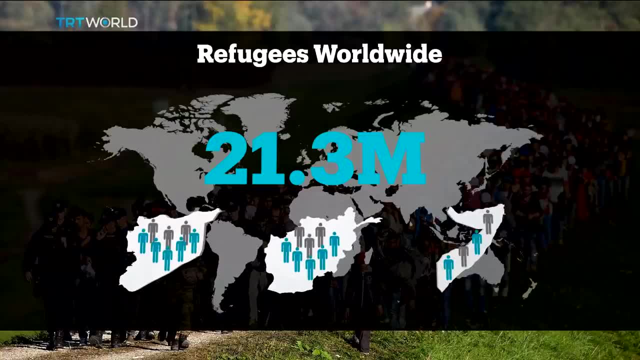 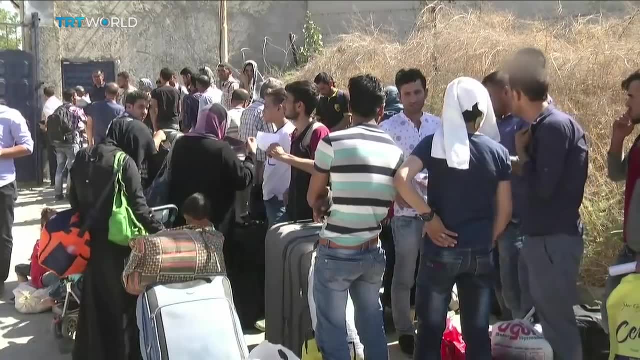 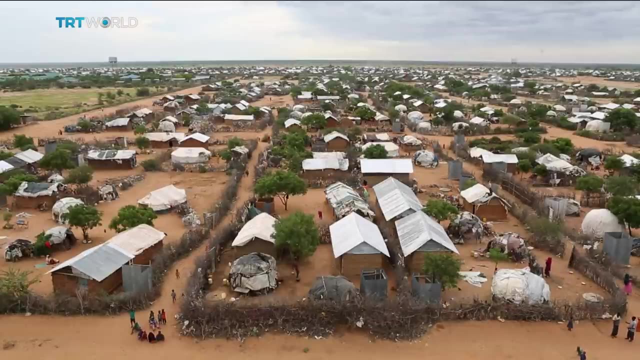 three countries: Syria, Afghanistan and Somalia. One of the few bright spots this year: Thousands were able to return to the Syrian city of Jarabulus after Turkish forces took it from Daesh. But there are still few places in the world where refugees are made to feel welcome. 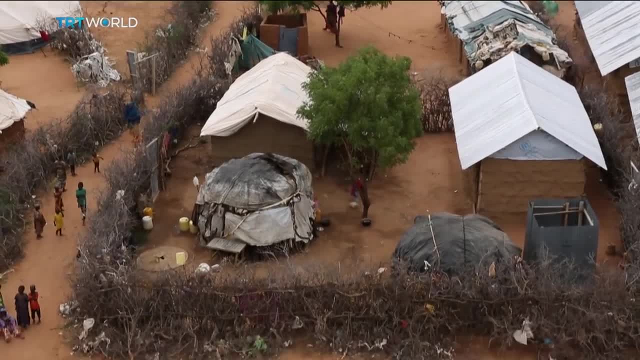 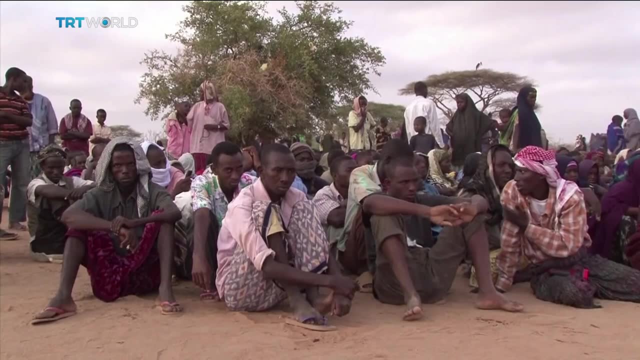 In Kenya, the largest camp in the world is due to be shut down next year. The Darb is home to hundreds of thousands of Somalis And it's a potential security threat, according to the authorities. Andrew Hopkins, TRT World. Transcription by ESO. Translation by —.